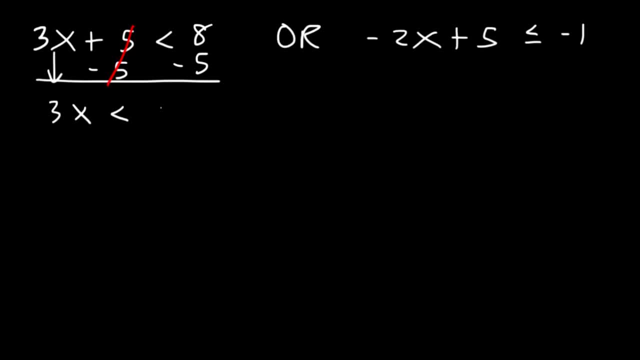 3x and 8 minus 5 is 3.. Next let's divide both sides by 3. So we can see that x is less than 1.. Now for the other side. let's begin by subtracting both sides by 5.. 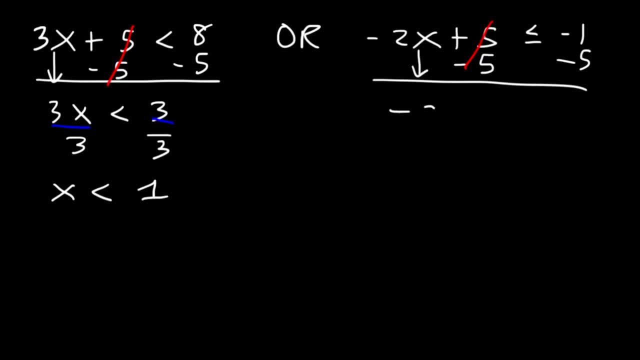 So what we now have is: negative 2x is less than or equal to negative 1 minus 5,, which is negative 6.. Now, just like we did before, we need to divide both sides by the number in front of us. We're going to multiply both sides by 4.. We're going to write the equation for: 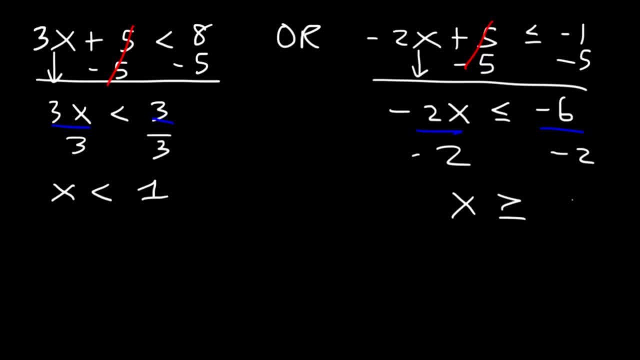 2x plus 3x plus 4.. We're going to call it the ш, and what we're going to do is divide 2 equal to 4, and here's our number line from the surface. So let's put in 4, or motion on. 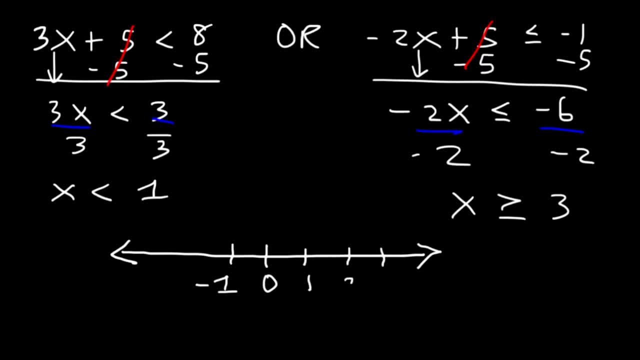 the surface, 2, and 3.. Now, x is less than 1, but not equal to it. So we're going to have an open circle and because it's less than, we're going to shade towards the left. 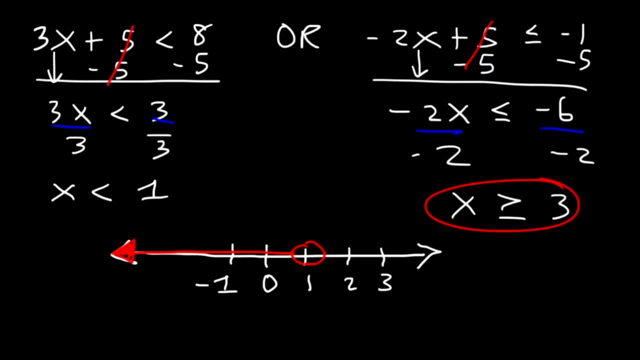 Now, x is also greater than or equal to 3.. Because we have the underline, because it can equal 3,, we're going to have a closed circle at 3.. And because it's greater than, we're going to shade it towards the right. So that's how you can graph the solution, using a number line. Now, 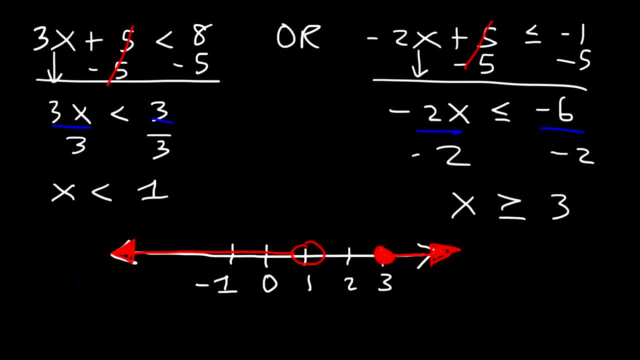 how can we write the answer? using interval notation? All the way to the left we have negative infinity and all the way to the right we have positive infinity. So the answer, the first part, is going to start from negative infinity to 1.. 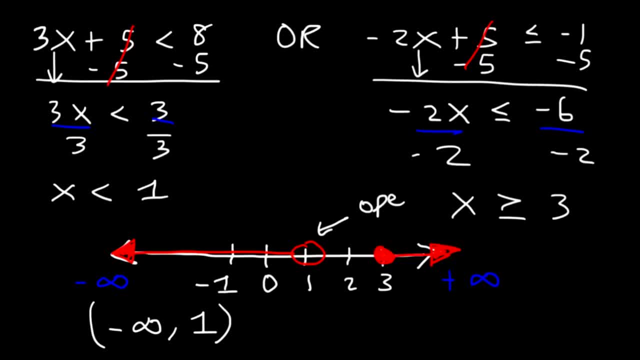 Now, whenever you have an open circle, make sure you use parentheses as opposed to brackets. Now, at 3,, 3 is included, so that's a closed circle. We need to use brackets. So that's the answer. using interval notation. 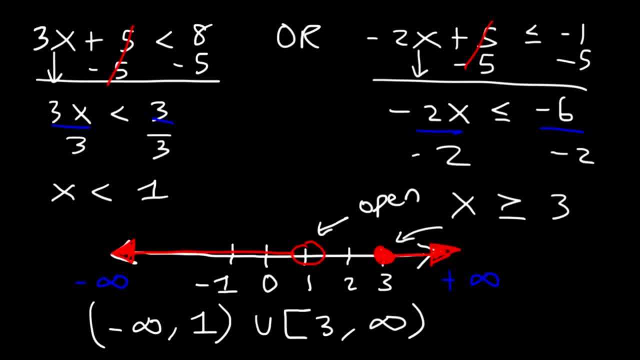 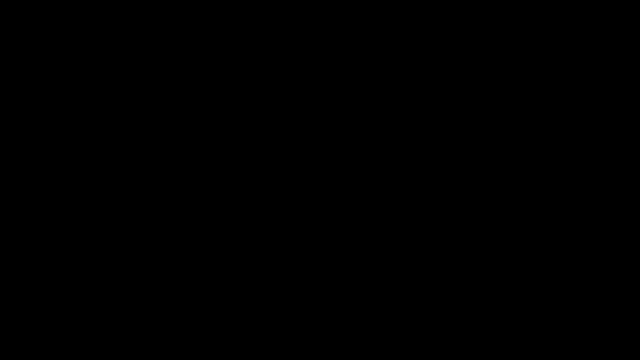 x could be anything between negative infinity to 1, but not including 1, and anything between 3 and infinity, including 3.. Here's another problem that we could try. Let's say that 7 is less than 1, but not equal to it, So we're going to have a closed circle. 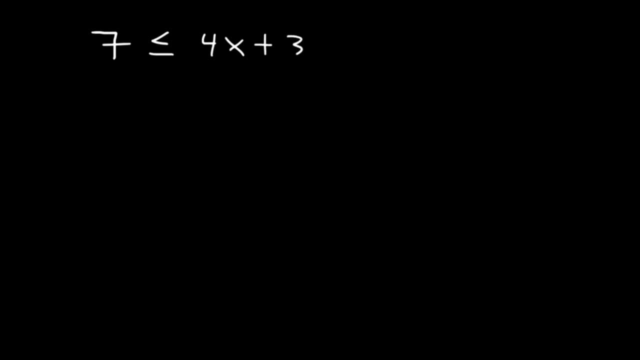 less than or equal to 4x plus 3,, which is less than 23.. So here we have another compound inequality. The other one was associated with the word or and this one's associated with the word, and Go ahead and solve it. Feel free to pause the video. 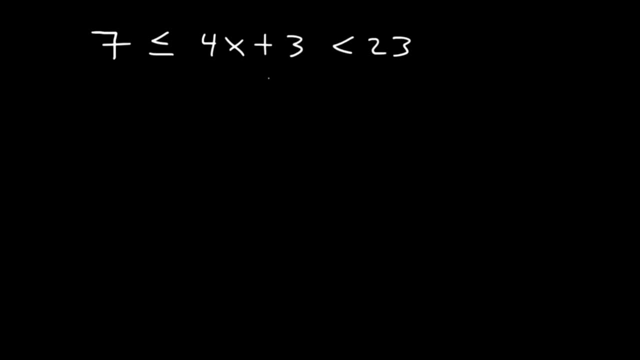 So what's the first thing that we should do in this problem? The first thing that we can do is subtract all three sides by 3.. If we do that, this is what we're going to get. 4x is greater than 7 minus 3, which is 4,. 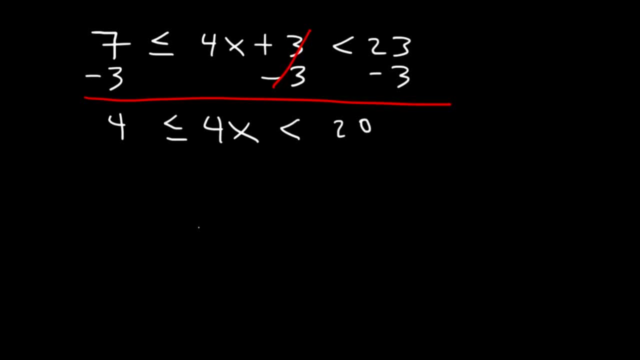 and it's less than 23 minus 3, which is 20.. Next we can divide all three sides by 4.. Our goal is to get x by itself in the middle. So 4 divided by 4 is 1, and 20. 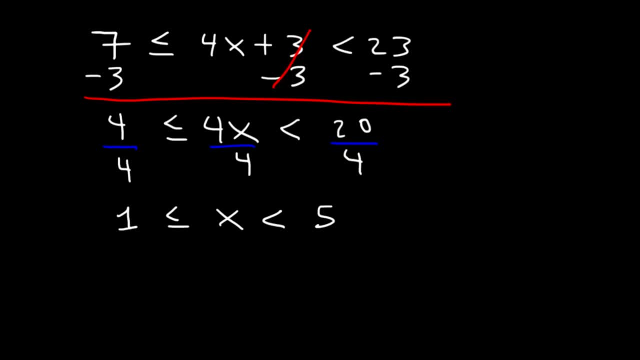 divided by 4 is 5.. So x is between 1 and 5.. Now let's plot this on a number line. Now, at 1,, should we have an open circle or should we put a closed circle? Notice that x is equal to. 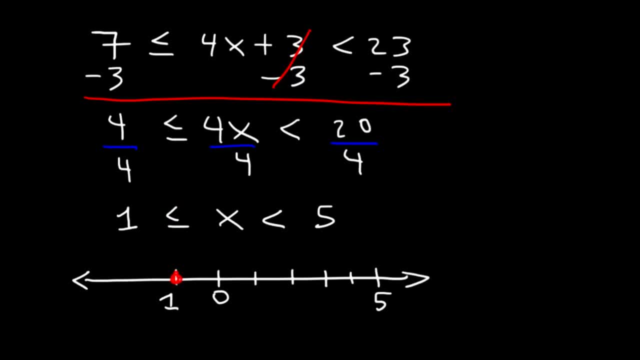 or greater than 1.. So it includes 1.. Therefore, we need a closed circle at 1.. And because it's greater than 1, we need to shade towards the right. Now, looking at the other side, x is less. 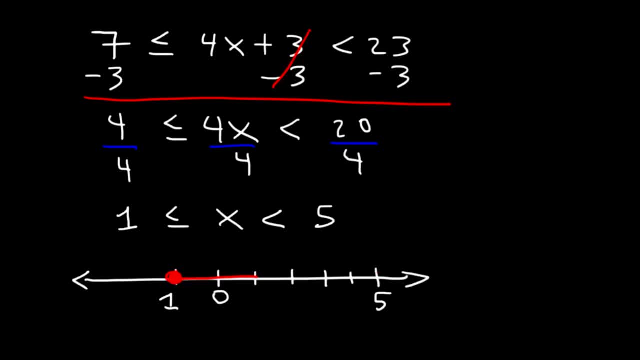 than 5, but not equal to it. So we're going to need an open circle at 5.. And because it's less than 5, we need to shade towards the left And we can clearly see that x is between 1 and 5.. 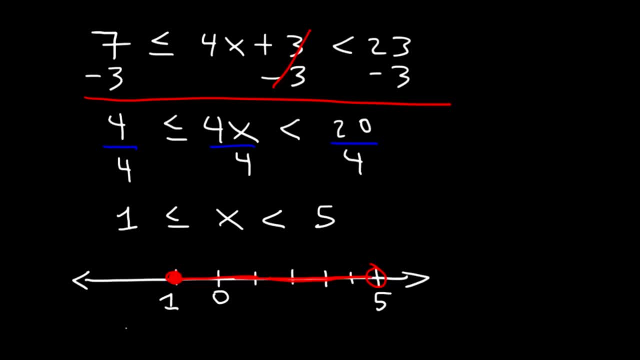 Now how can we represent the answer using interval notation? Starting at 1, we need to use a bracket And then after that it stops at 5.. But because we have an open circle at 5, we need to use parentheses. So that's the answer using interval notation. It's. 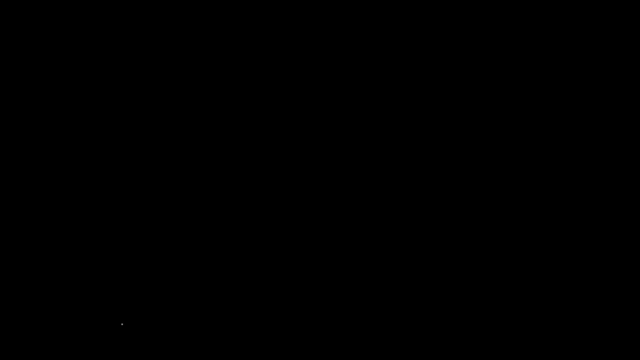 simply from 1 to 5.. So now here's another problem that you could try. 1 third x plus 2 is less than, or equal to 4.. Or 6 minus 2 over 5x is less than 2.. So take a minute, pause the video and try this example. 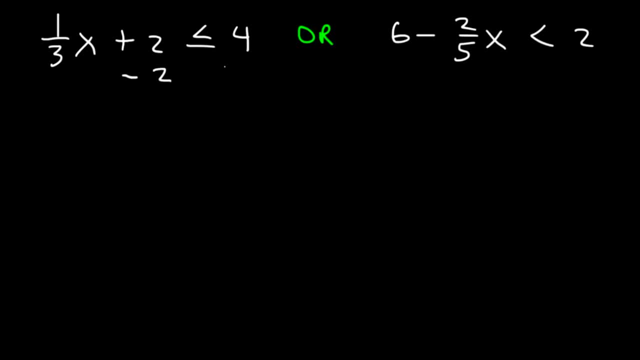 So let's start with the 1 on the left. Let's begin by subtracting both sides by 2.. So 1 third x is less than or equal to 4 minus 2, which is 2.. Now what should we do at this point to get rid of the x? I mean not the x, but to get rid of the. 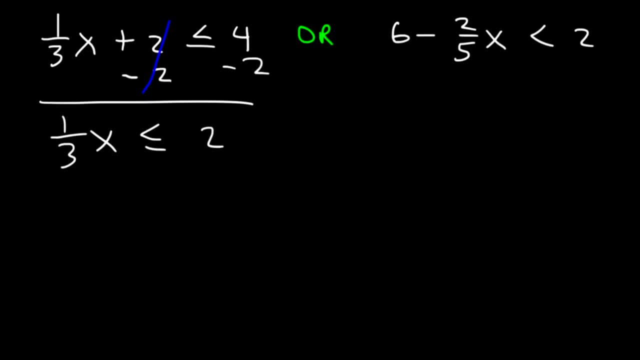 fraction. If you want to get rid of the fraction, multiply both sides by 3.. 3 times 1, third, which is 3 divided by 3, that's equal to 1.. Or 1x, which is simply x. 2 times 3 is 6.. So x is less. 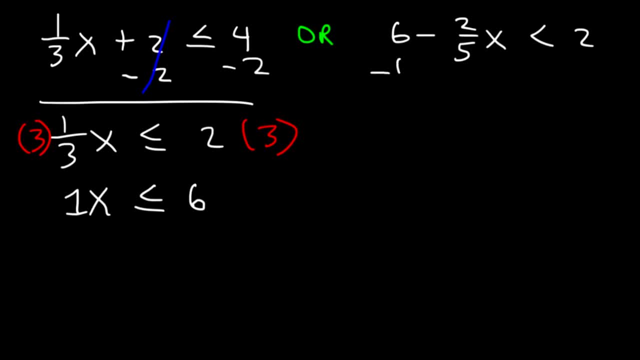 than or equal to 6.. Now for the other one. let's begin by subtracting both sides by 6.. So now we have negative. 2 over 5x is less than 2 minus 6, which is negative 4.. So now, 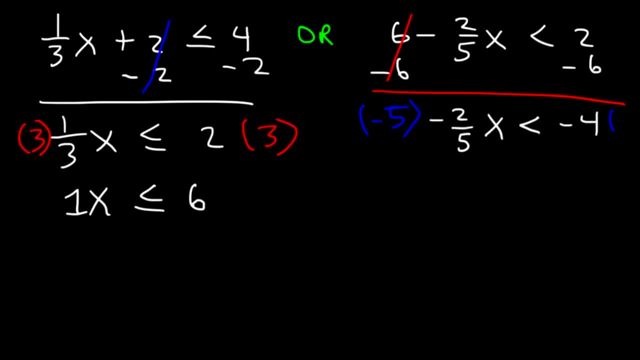 let's multiply both sides by negative 5. And keep in mind: any time you multiply or divide by a negative number, the inequality will change direction. So these will cancel and we're going to have positive 2x on the left side and that's greater than negative 4 times. 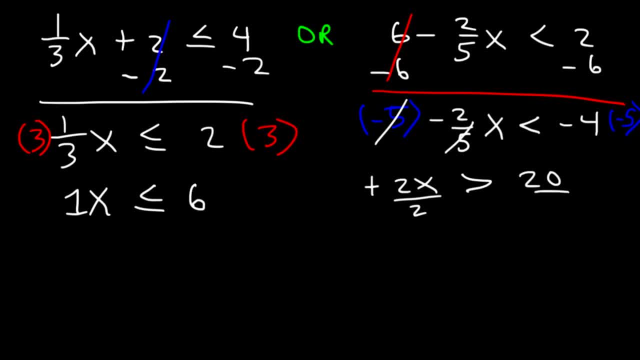 negative 5,, which is positive 20.. Now let's divide both sides by 2.. x is greater than 10.. So let's say this is 6, and this is 10. And we have the numbers in between. So x is equal to or less than 6.. So we're. 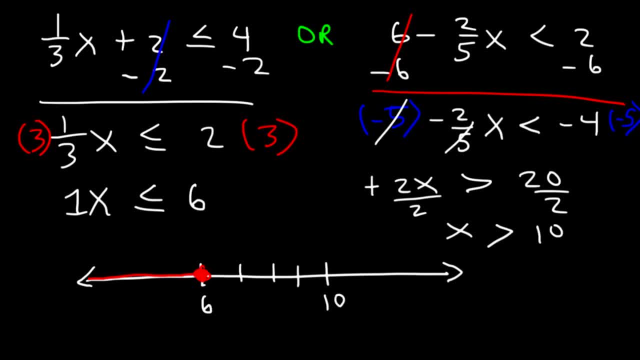 going to have a closed circle at 6.. And because it's less than, we're going to shade towards the left. x is greater than 10, but not equal to it, So we have an open circle shaded towards the right. At the right, we have positive. 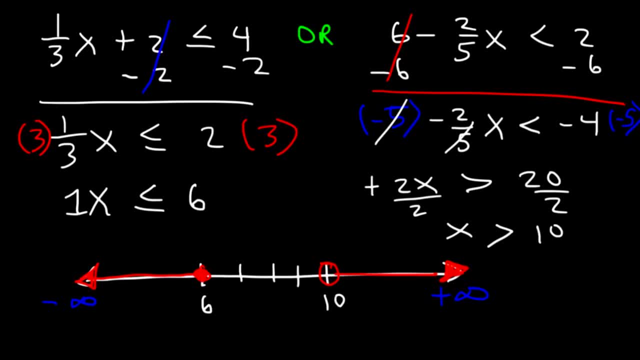 infinity and at the left, negative infinity. So the answer, using interval notation, is negative infinity to 6, since it includes 6.. We're going to use a bracket because we have a closed circle, And then union 10 to infinity Any time you have an open circle. 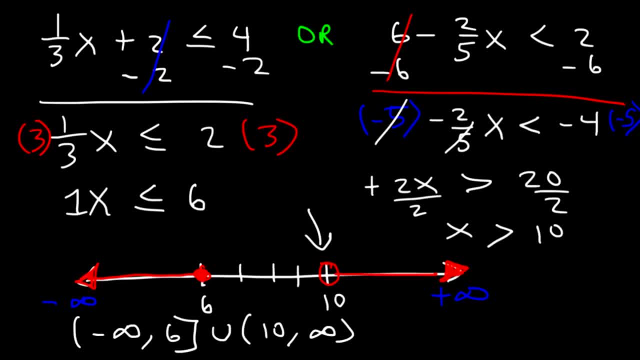 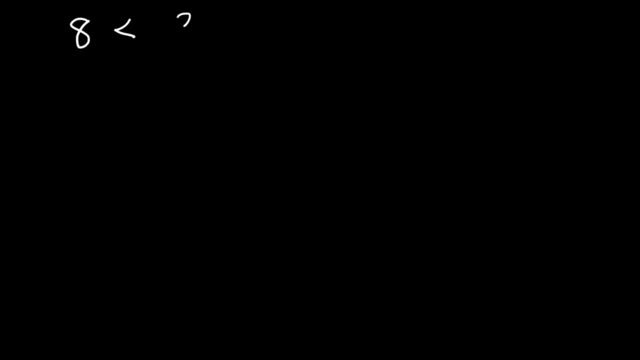 make sure you use parentheses. So for infinity symbols you should always use parentheses. Here's another one that we could try: 8 is less than 2 over 3, x plus 6, which is less than or equal to 12.. Try that one, Find a solution, plot it on a number line and then. 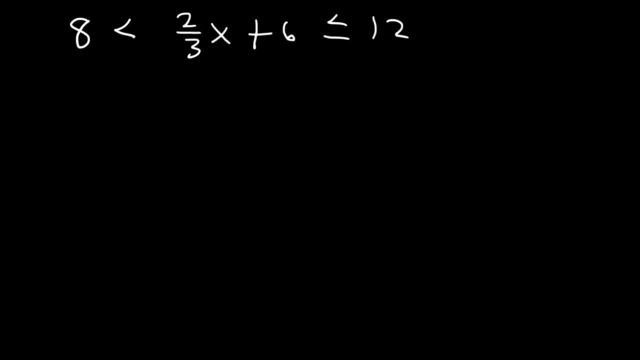 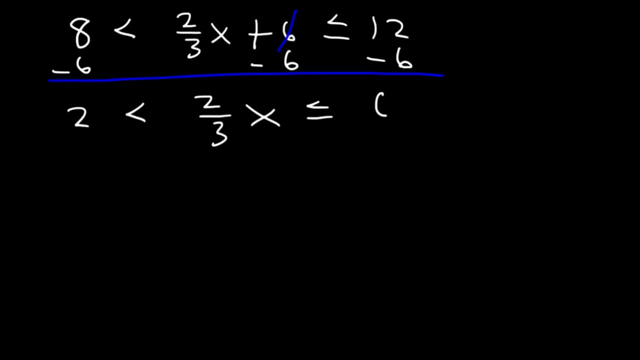 8 minus 3 x plus 6.. 8 minus 3 x plus 6.. 9 out of 10.. 9 out of 10.. 10 minus 6 is 2.. 12 minus 6 is 6.. 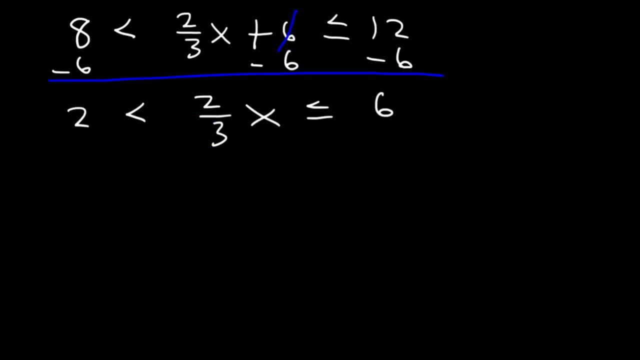 Now we have a fraction, so let's multiply both sides by the denominator of the fraction. So we're going to multiply all three sides by 3.. 2 times 3 is 6.. 3 times 2 thirds: the 3's will cancel, leaving behind 2 x. 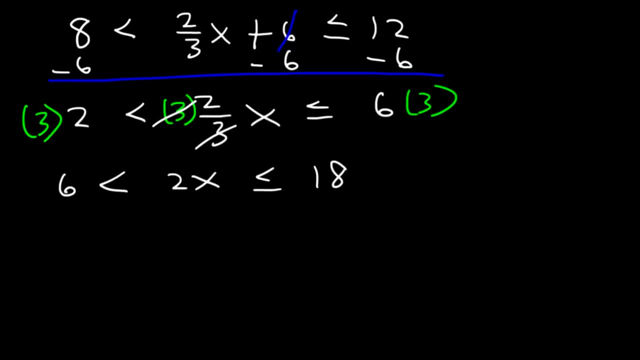 6 times 3 is 18.. Next, 6 times 3 is 18.. 3 sides by 2.. 6 divided by 2 is 3.. 2x divided by 2 is just x. 18 divided by 2 is 9.. So x. 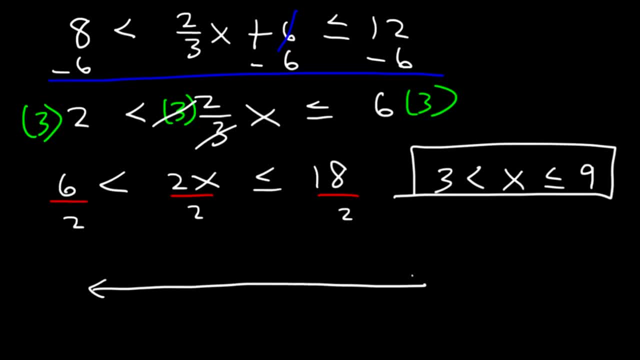 is between 3 and 9.. So let's say this is 3 and this is 9.. Now x is greater than 3, so it doesn't equal 3.. So we have an open circle shaded towards the right. x is less than or. 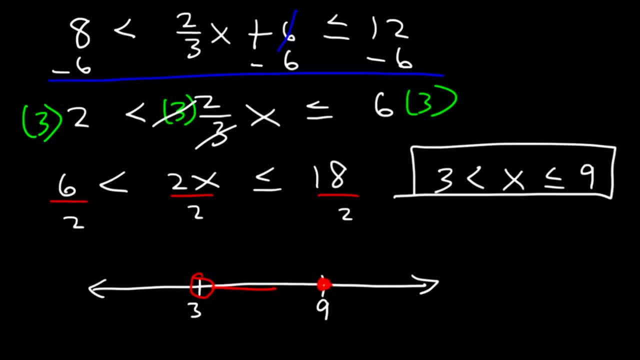 equal to 9.. So it's a closed circle at 9, shaded towards the left. So it's between 3 and 9.. And in interval notation the answer is going to be 3 to 9, but with a bracket at 9, since 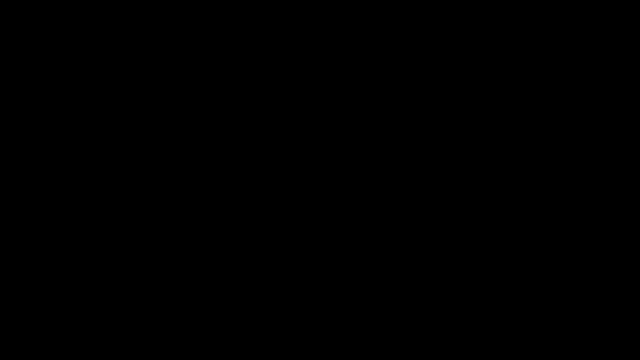 we have a closed circle at 9.. So that's it for this video. Thanks for watching. By the way, if you want to find more videos, you can check out my website. I'll put a link on my website, video-trudanet, Or you can go to my channel and you can find playlists. 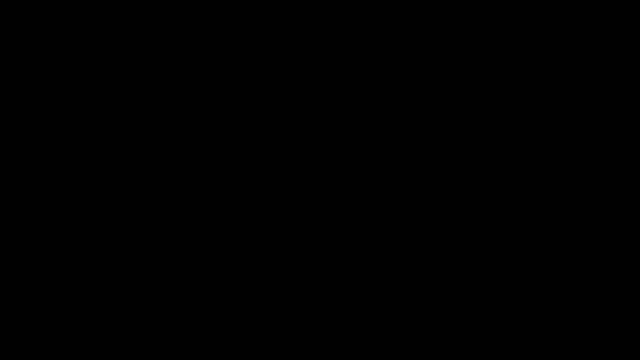 on algebra trig, precal calculus, chemistry and physics. So go ahead and take a look at those, and thanks again for watching this video. 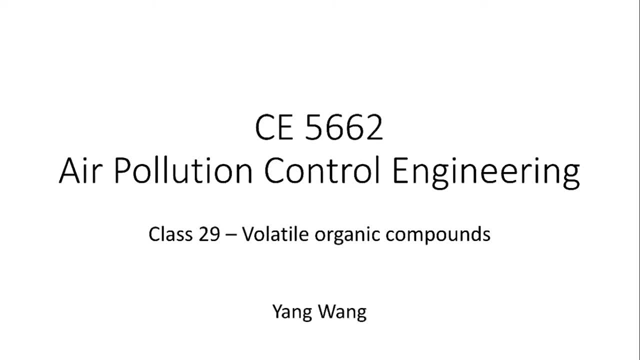 So I sent a mid-semester review after our last class. I think this is what our department recommends for the new faculties, because I just joined last year and this is the second time I'm opening this class, So any feedback is highly appreciated. I don't think that's. 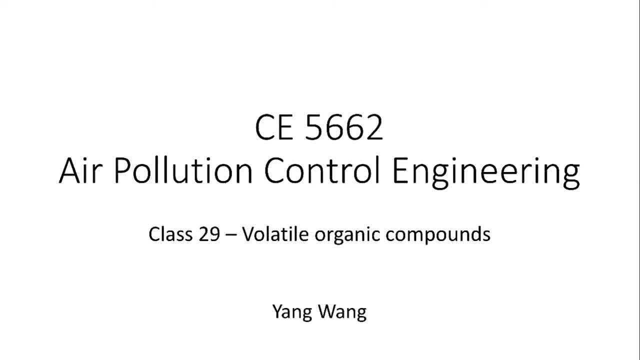 a very long survey. So I would say, maybe after this class you can spend some time to go through the questions and then just leave some comments, right? No matter whether it's good or bad, right? So I think the major comment I got from our last year was that 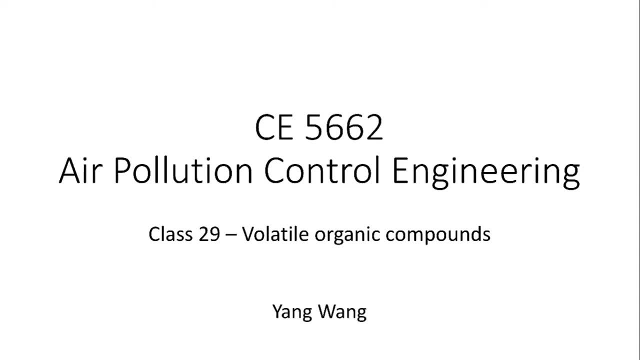 people were complaining the term projects are too close to the presentation. So basically, for last year the sulfur dioxide was taught maybe in the last month of the whole semester, So some students were feeling that they don't have enough time to go through the contents. So this year we're moving the sulfur oxides, or nitrogen oxides, to earlier. 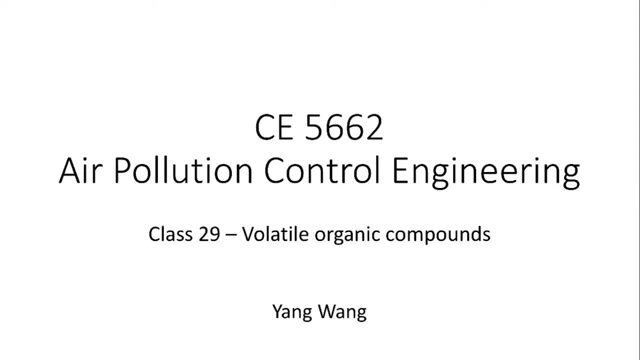 of the semester, So I hope this can give you guys more time to work on the project. So I also got some feedback from a few groups about content. So I hope this can give you more time to work on the project. So I also got some feedback from a few groups about